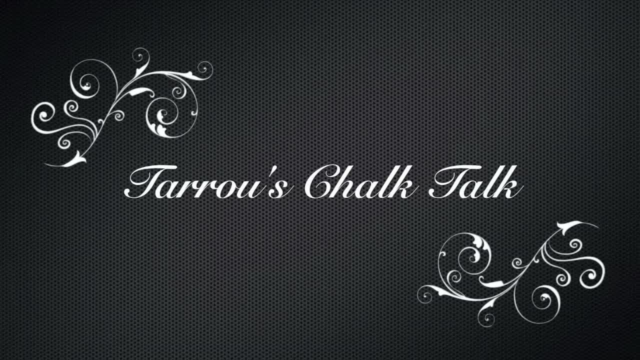 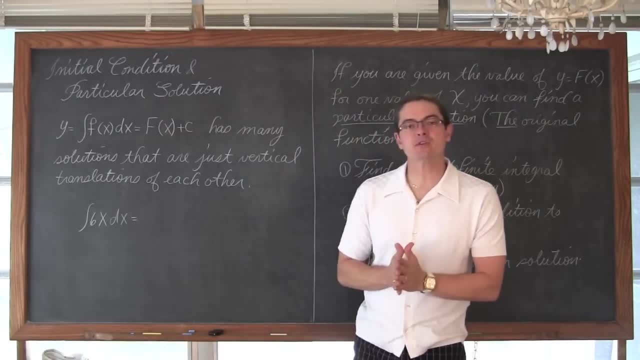 BAM, Mr Tarrou. Ok, we are in part 2. here We are going to expand our introduction of finding antiderivatives and the indefinite integration process by showing you how to use an initial condition to find a particular solution. Now, what I mean by that is: we have 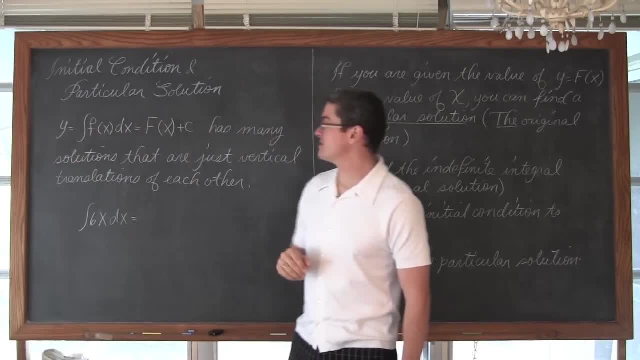 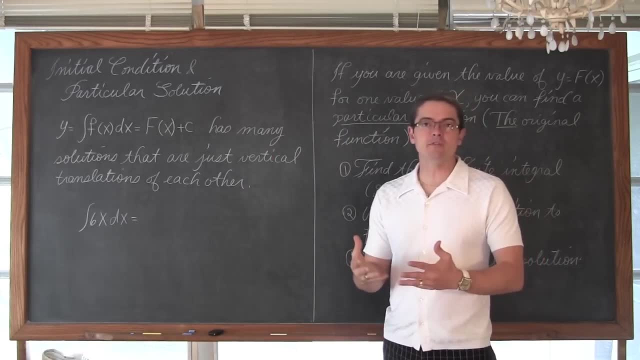 here, y is equal to the antiderivative of f of x with respect to d, and that is equal to f of x plus c. We talked about how, when we do find an antiderivative from a derivative, if that is all we are given, is that derivative? then, remembering that the derivative of a 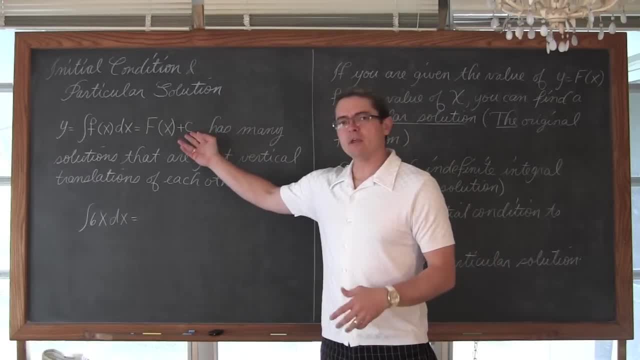 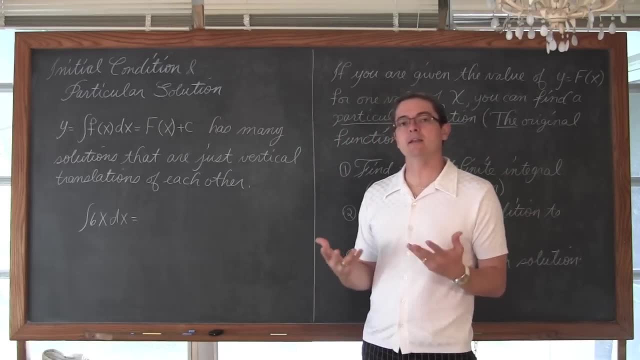 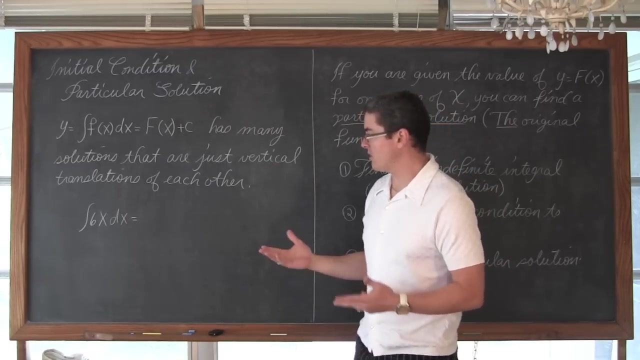 constant is zero. when we find that antiderivative, we don't really understand or we don't have enough information to find out what c is. So there are many, many solutions when you find an antiderivative. All of those solutions are just simply vertical translations of themselves. So again, the 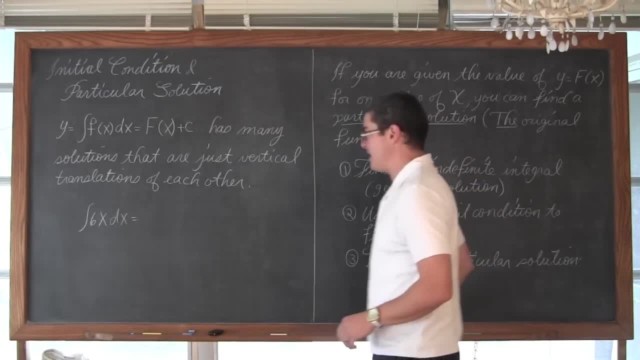 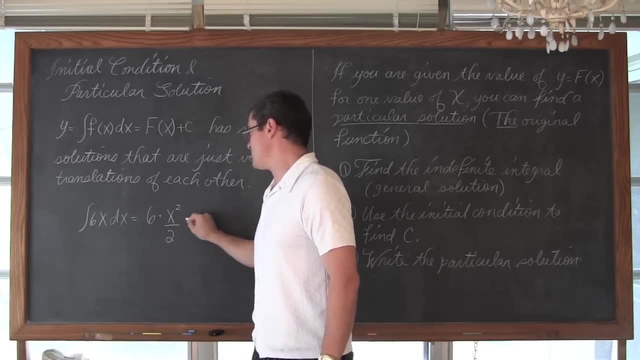 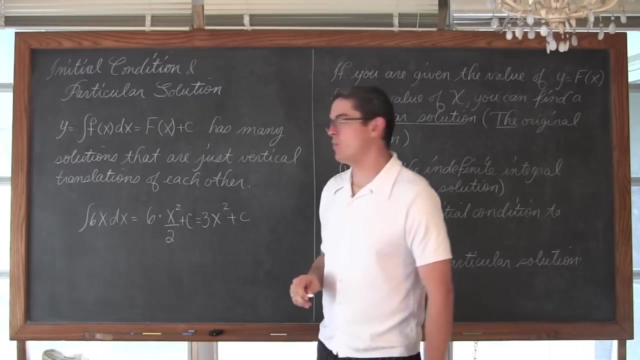 antiderivative of 6x with respect to x is going to be equal to 6 times x squared divided by 2, which is equal to 3x squared plus c. I should have added that plus c here as well. So we have f of x is equal to 3x squared plus c. So we have f of x is equal to 3x squared. 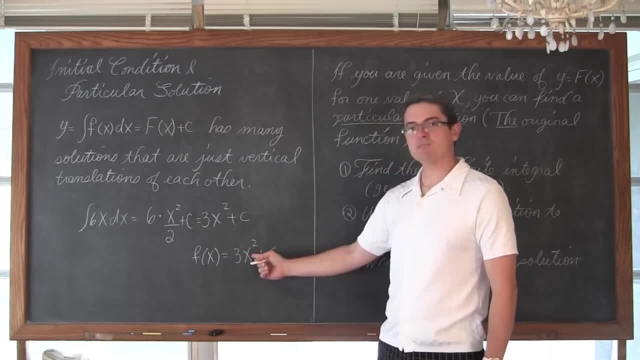 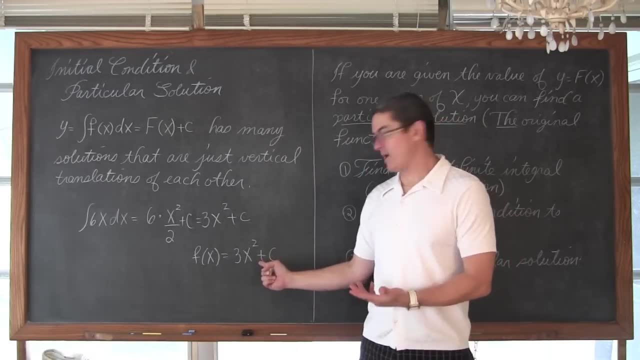 plus c. So I don't know if this parabola- oh, excuse me, someone got my little dog barking there- I don't know if this parabola. this has a power of 2, so I don't know if this. 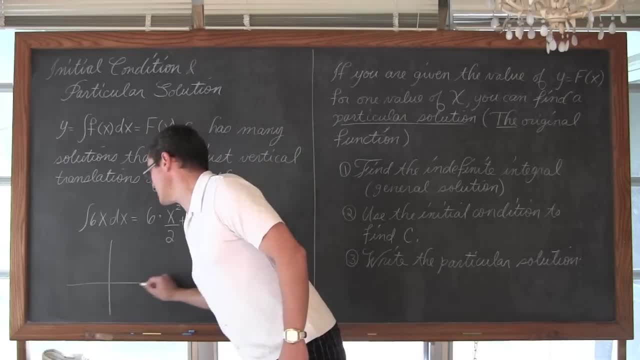 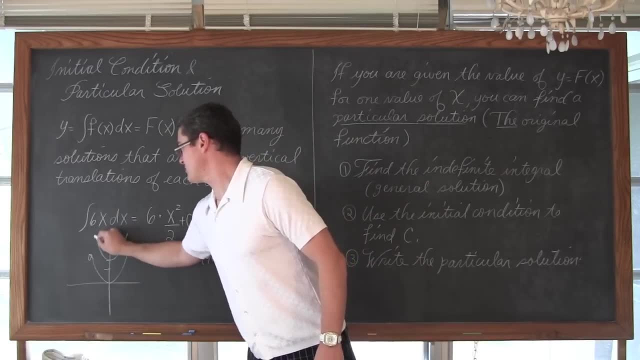 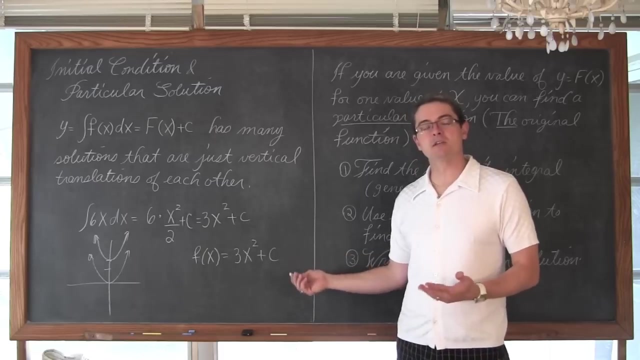 parabola passes through the origin, or maybe this parabola had a vertical shift of 2 and thus passed through the point of, along with many other points, of course. You know I'm a plus c, I have a constant at the end. So while I know the family of antiderivatives, 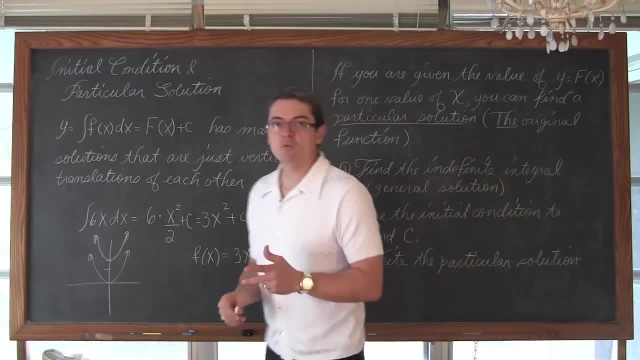 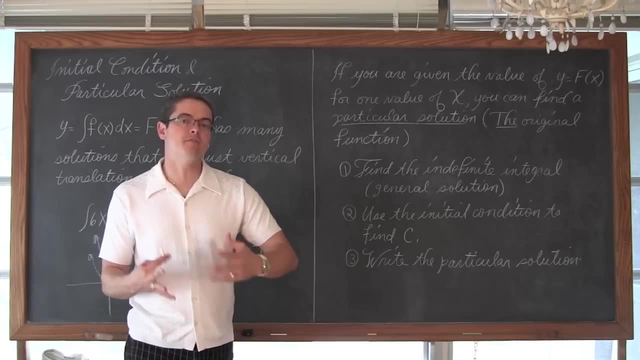 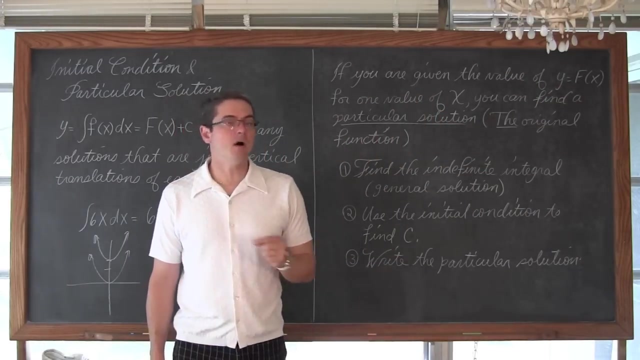 I don't know the solution. Now, if we are given just a little bit of information beyond the derivative that we are finding the antiderivative of, we can actually find the original function. If you are given the value of y equals f of x. for one value of x you can find a particular 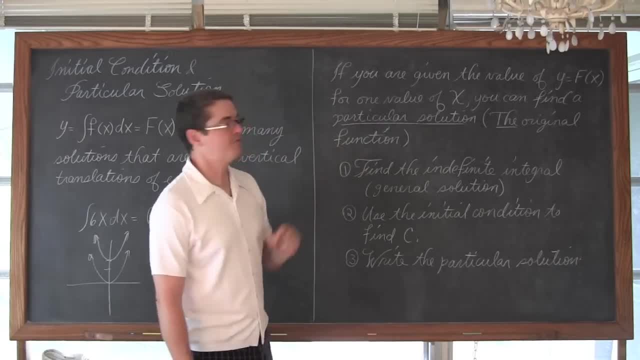 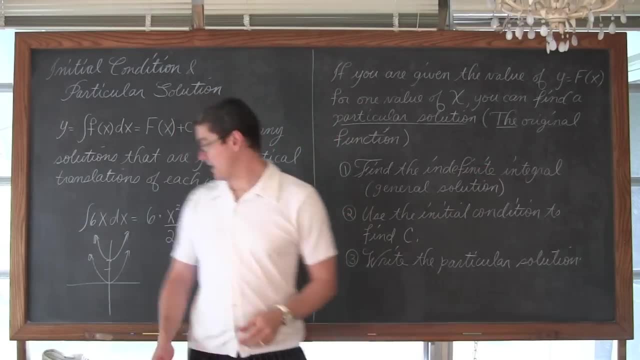 solution, The one original function for the original function of x. So if you are given the conditions that are given to you in your problem, what you are going to do is first find the indefinite integral. that general solution, like I have here with my f of x, is: 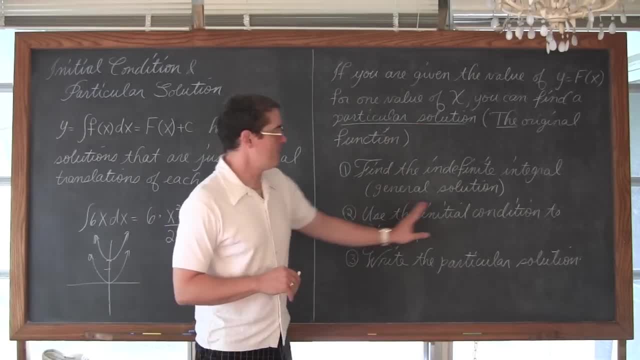 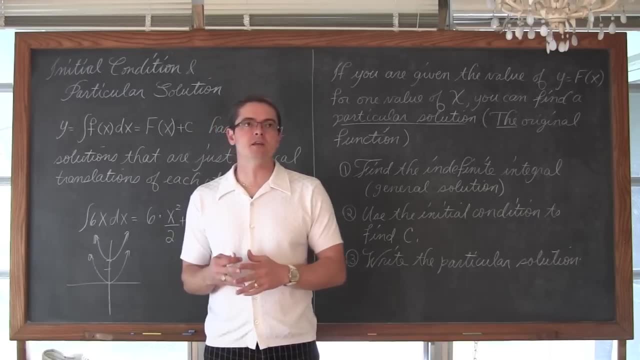 equal to 3x squared plus c, You are going to use the initial condition to find c. In other words, the problem- and I'm not going to finish this one, but the problem will say: okay, the original function is equal to 10 when x equals 2, something like that We are. 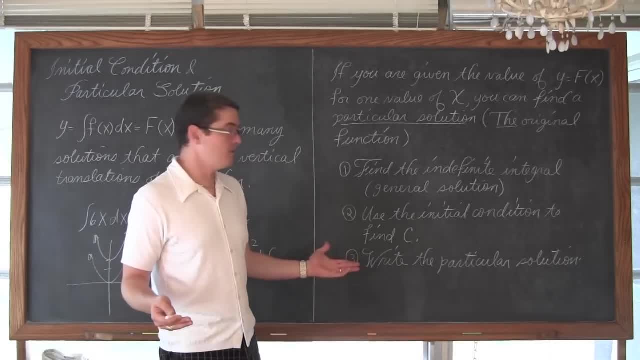 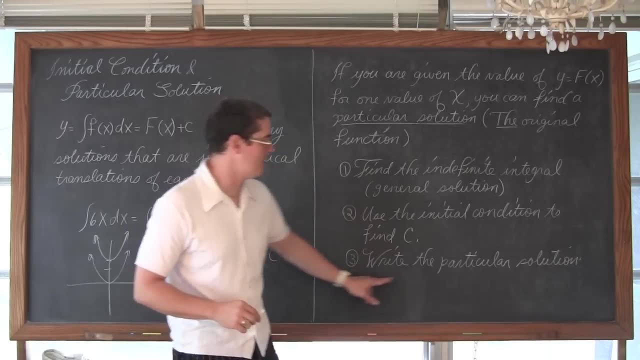 going to plug those values in, find the value of c, and then you know, with that specific given, you know that one little point, that the graph, the function, actually passes through, we will find c and then be able to write our particular solution. We are going to do: 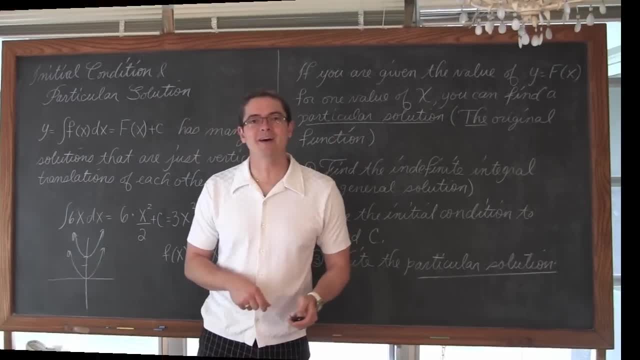 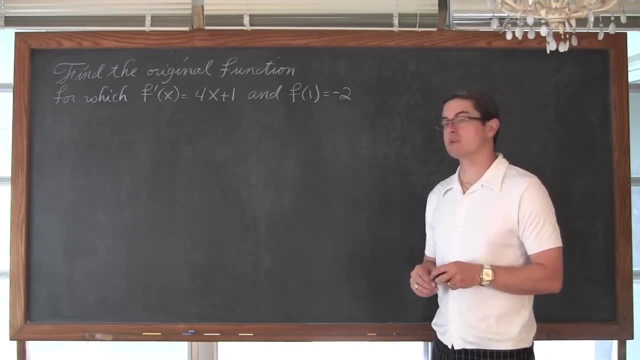 two examples. so this will be a fairly quick video and let's get to them right now. So we have the problem find the original function for which f prime of x is equal to 4x plus 1, and f of 1, so this prime symbol is gone now. so we are talking about the original. 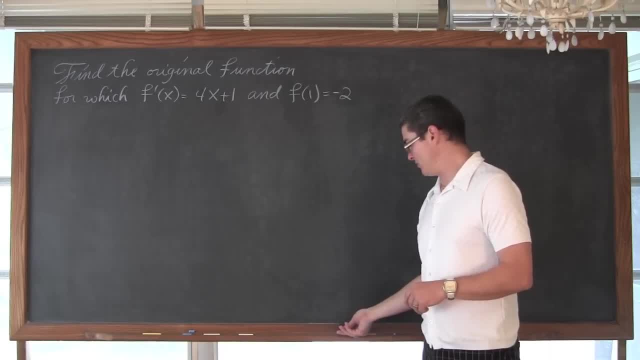 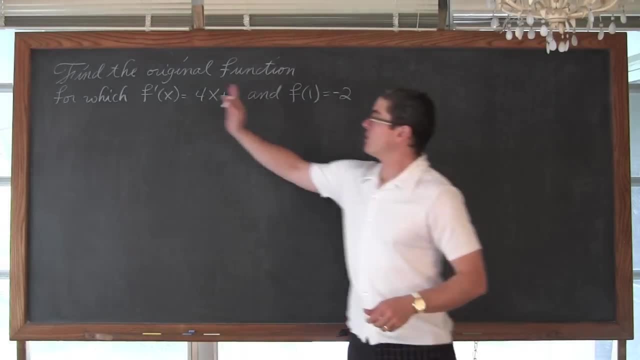 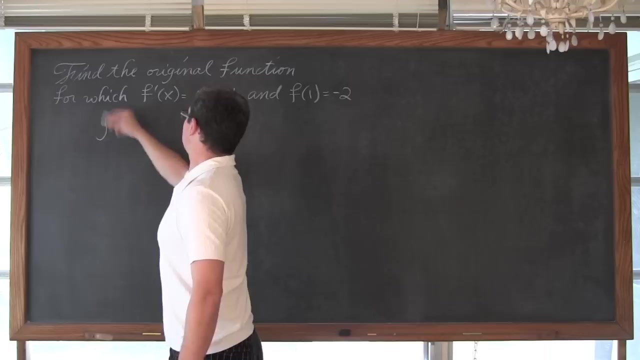 function f1 is equal to negative, 2.. So, of course, first we need to find the antiderivative, We need to do the indefinite integration. for f. prime of x is equal to 4x plus 1. So we have the indefinite, the integral of 4x. 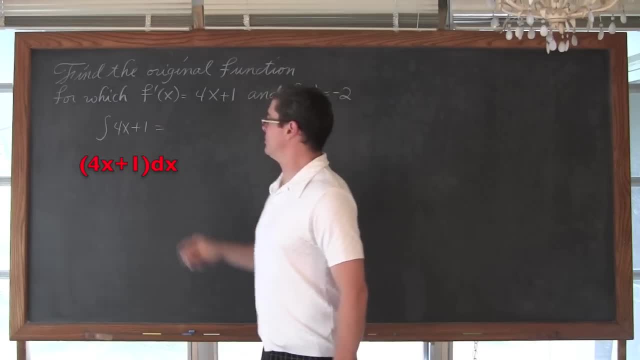 plus 1 is equal to 4, we are going to take that exponent of 1 and increase it by 1, so we have 4x squared 4 times x squared divided by 2, plus 4x squared divided by 2, plus 4x. 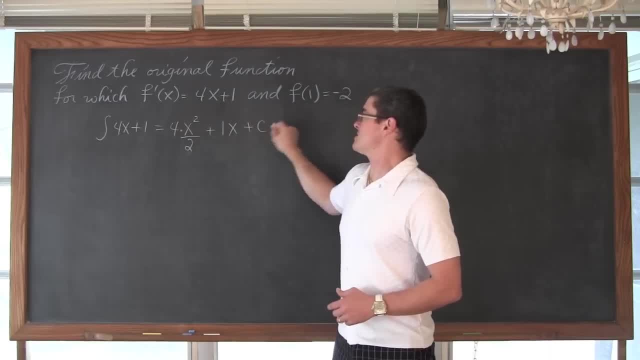 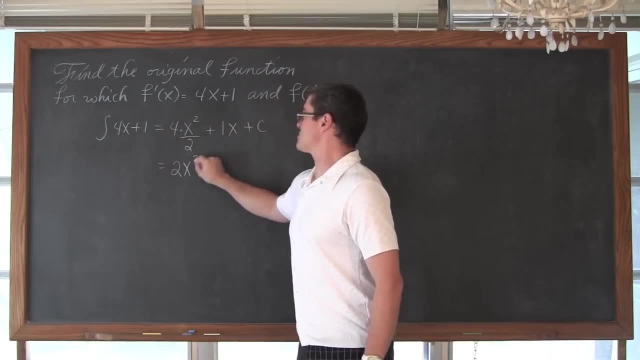 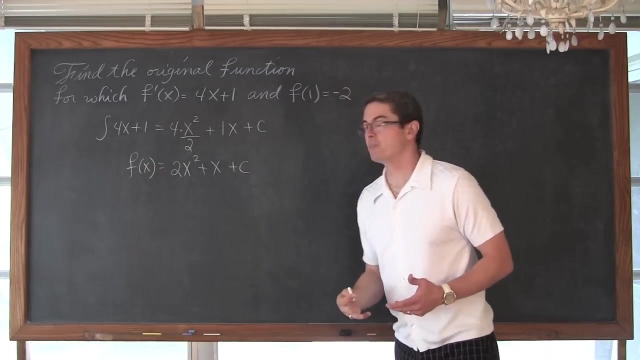 squared divided by 1x, And again, of course, plus c, because we are finding the general solution. So 4 divided by 2 is equal to 2x squared plus x plus c, and this is f of x, our antiderivative. Well, unlike my previous video, now we are given a little bit of extra. 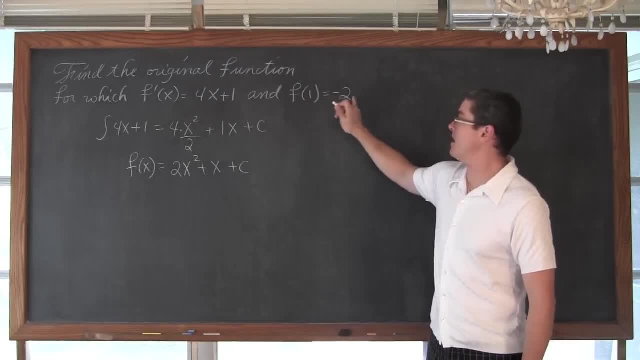 information. This function passes through the point of 1 comma, negative 2, or when x is equal to 1.. f of 1 or f of x is equal to negative. 2.. Plug into negative 1, or, excuse me, plug into 1,. 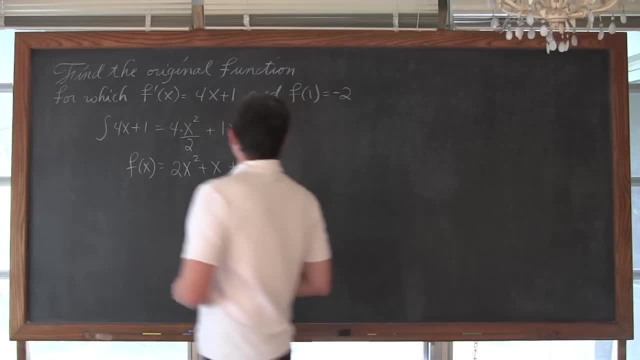 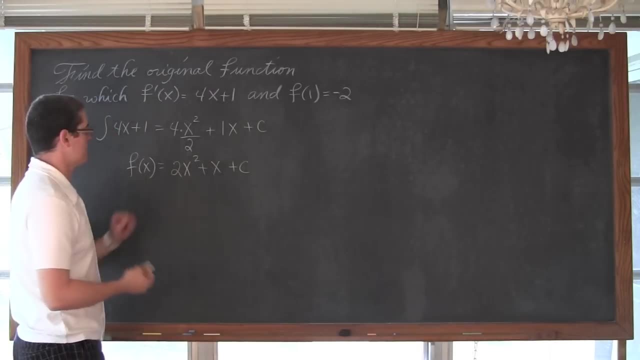 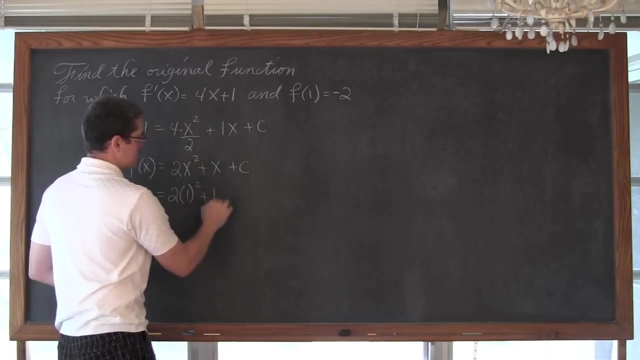 get out a y value of negative 2.. So what does that mean? That means that f of 1, when I take the value of 1 and plug it into this function, the overall value is going to equal negative 2.. So negative 2 is equal to 2 times 1 squared plus 1 plus c. So again I am plugging. 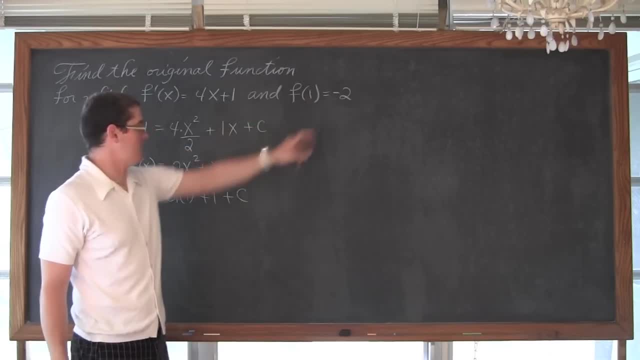 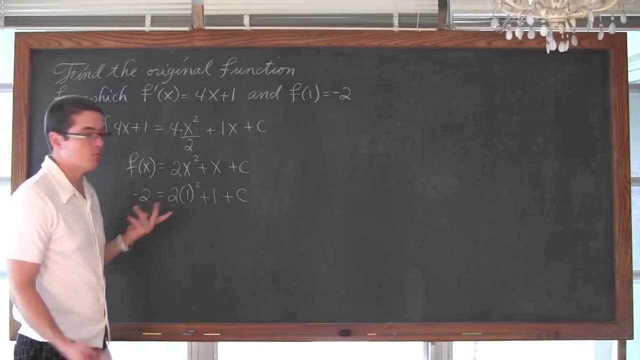 in my x value of 1.. When x is equal to 1, so the x's come out and 1 goes in their place- the entire function's value is equal to negative 2, or y equals negative 2.. So we have 2 times. 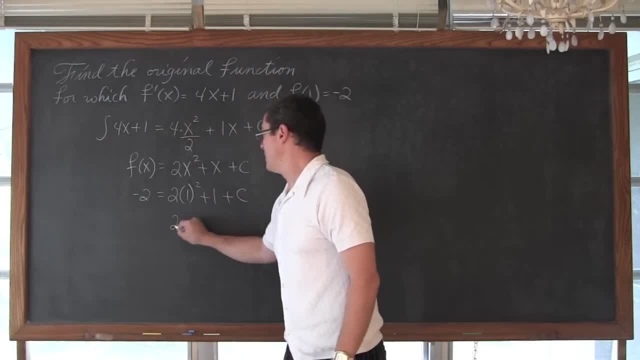 1 squared. well, 1 squared is 1, 2 times 1 is 2, plus 1 plus c is equal to negative 2.. That is negative. 2 is equal to 3 plus c. Subtracting both sides by 3, we get negative. 5 is equal. 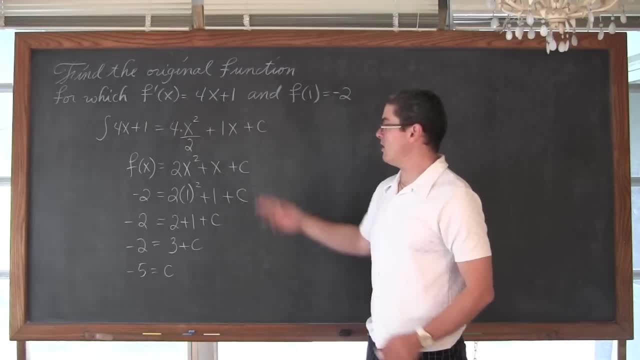 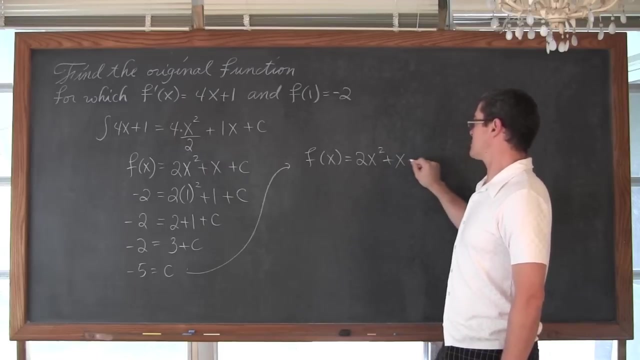 to c. So, unlike before, where all we could find was a sort of general solution, an antiderivative with an unknown constant, here at the end we have now our particular solution, the original function, And that is: using this value of c, f of x is equal to 2x squared plus x minus. 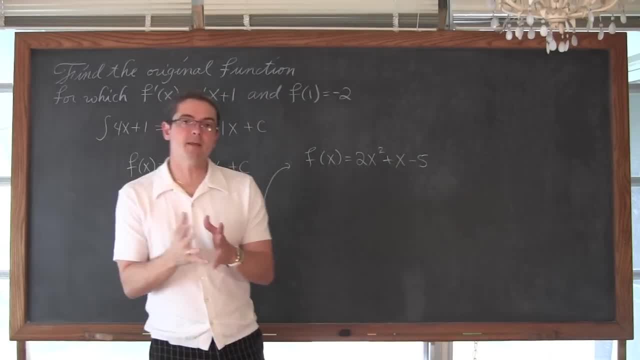 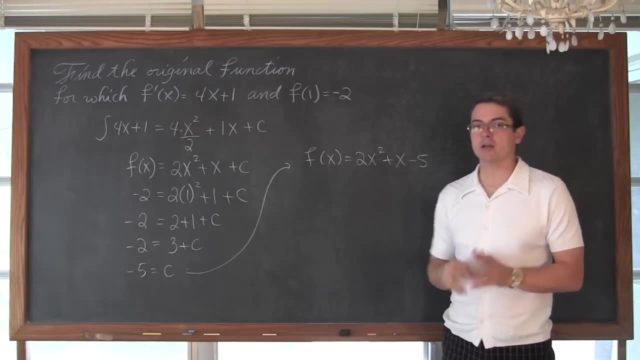 5. And that is pretty much all there is to it. We are going to find that antiderivative. we are going to take the initial condition, plug it in and find that particular solution. I have one more example. It is going to be a fairly straight forward algebraic example. 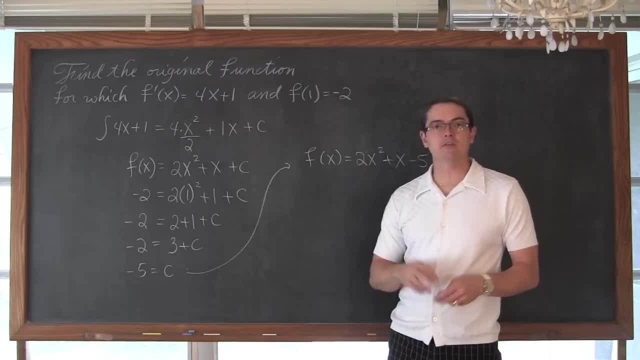 but they are going to be giving us the second derivative instead of just the first derivative, And that problem will simply need to be worked out in two parts as opposed to just one, Because we are going to have to find the antiderivative twice to go from the second derivative. that 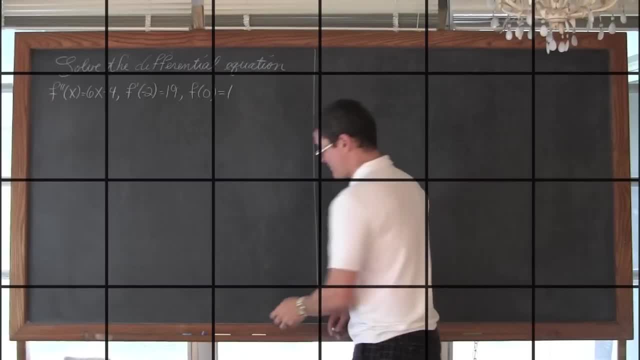 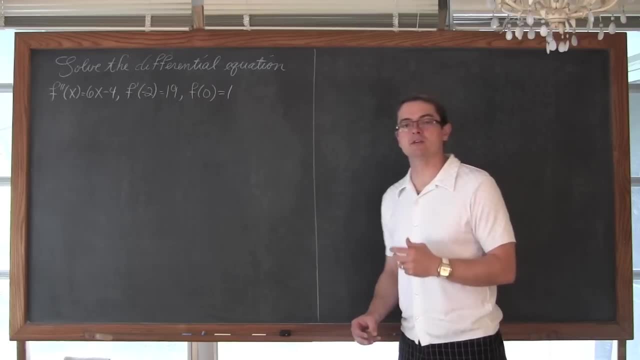 is going to be given to us, to the original function. Before we start our last example- I do apologize for getting that little dx notation at the end of my integral. I am going to use the original expression to say that we are finding the antiderivative with respect. 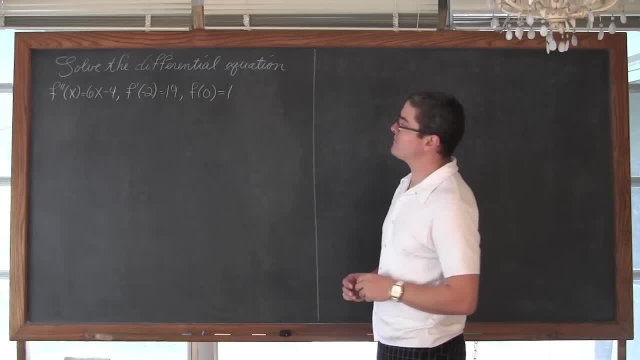 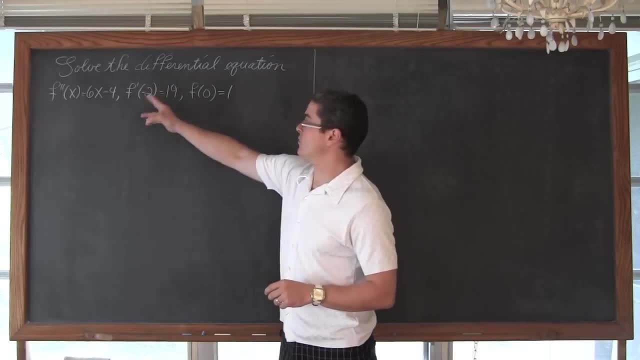 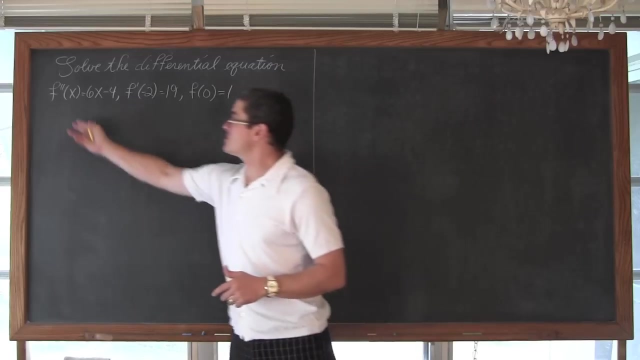 to x. Solve the differential equation: f double prime of x is equal to 6x minus 4,. given the initial condition for the first derivative, which is f, prime of negative 2 is equal to 19,. and then, finally, f of 0 is equal to 1.. Since we are given the second derivative, 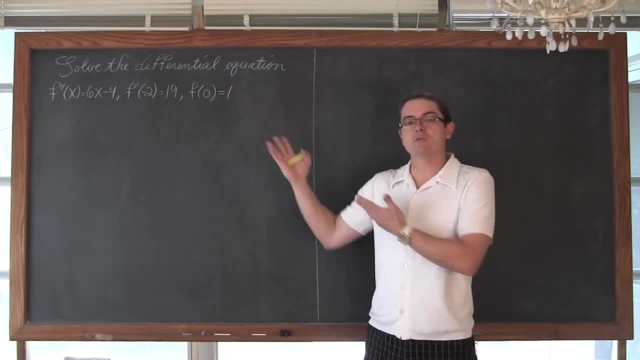 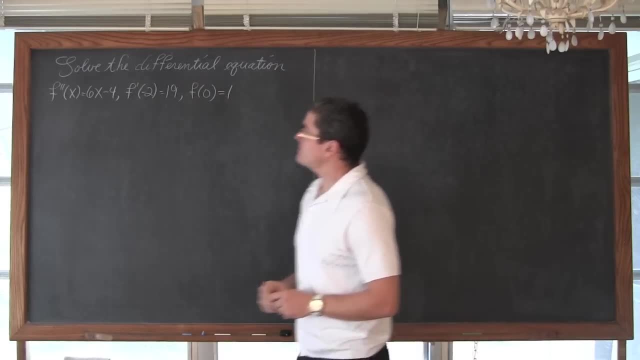 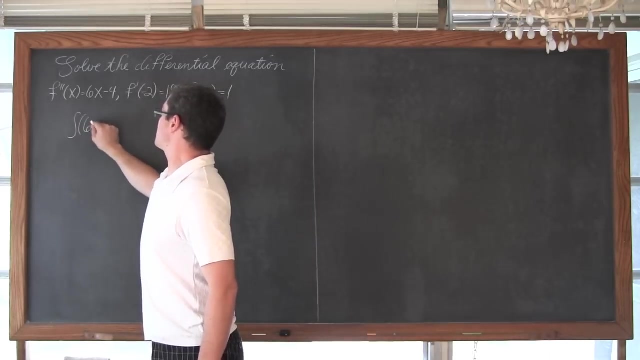 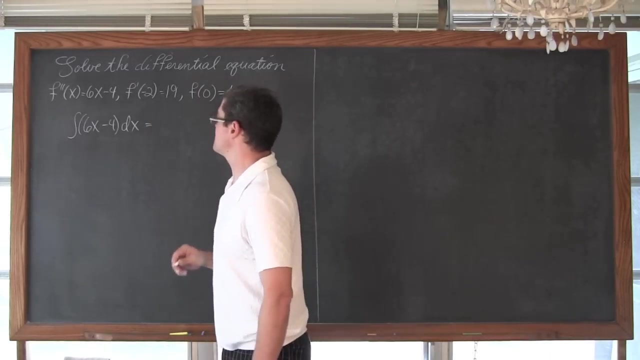 we are going to have to find the antiderivative twice to get back to the original function. It is the second derivative, so we have to do the antiderivative twice. We are going to find the antiderivative of 6x minus 4 with respect to x. That is going to give us 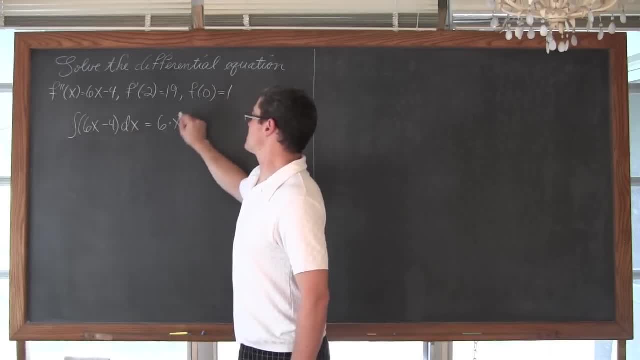 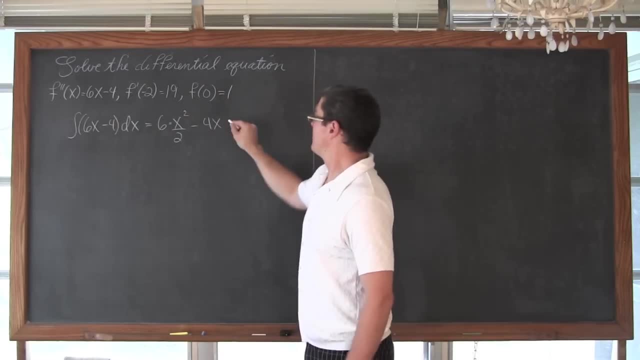 Let's see here. It is going to give us 6 times x squared divided by 2, minus 4 times x. We are going to raise: well, just times 4x plus c, We can find that general solution. Then 6 divided by 2 is equal to 3x squared minus. 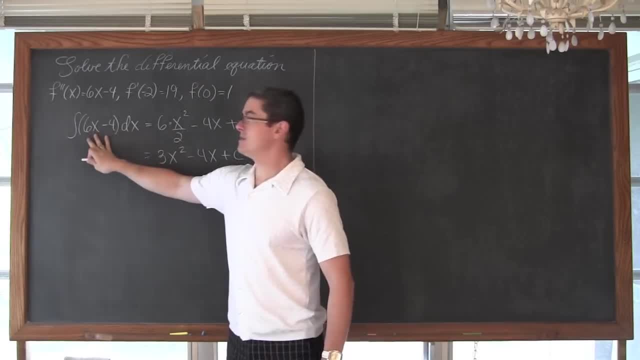 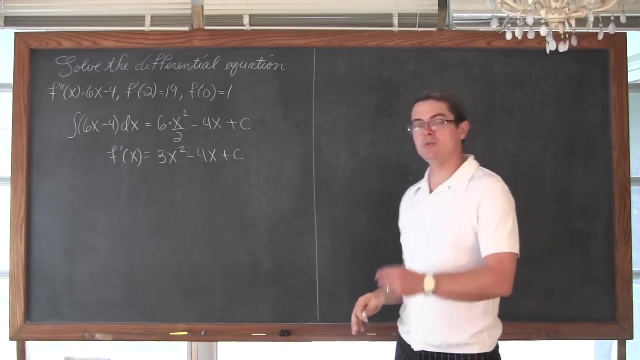 4x plus c. Now we started with the second derivative and found the antiderivative of that second derivative with respect to x, which means that if this was f double prime of x, then this is f prime of x. Again, that general solution. We are going to use the 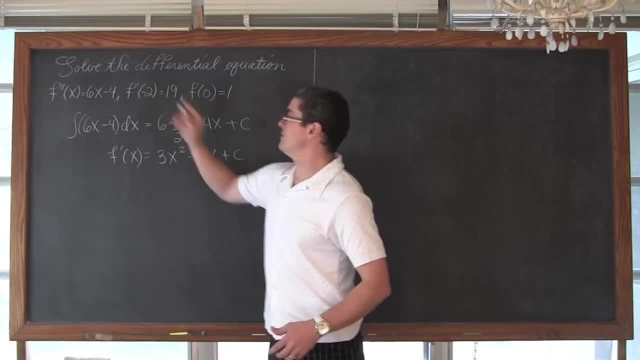 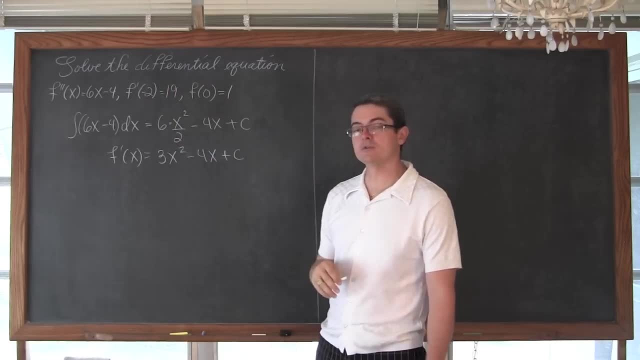 initial condition for the first derivative. It says that when x is equal to negative 2, the entire function, the entire first derivative, is equal to 19.. Plug in an x value of negative 2 and get a y value of 19.. So f prime of x. 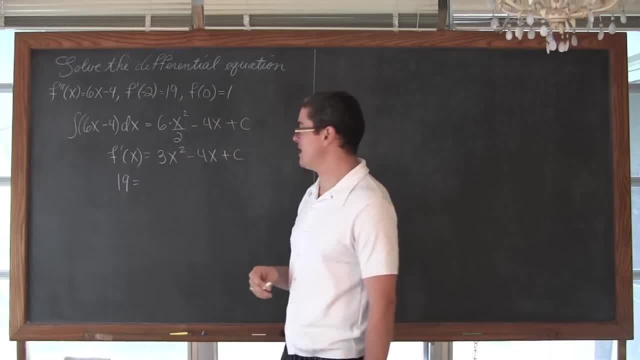 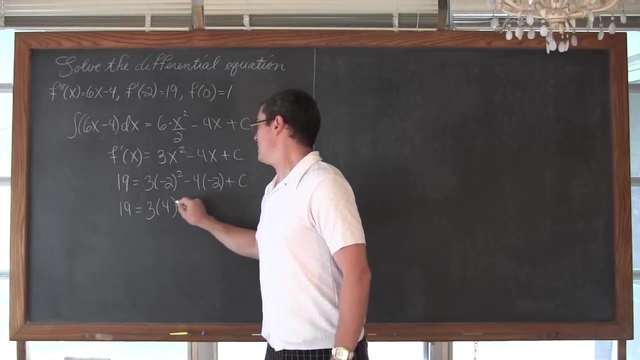 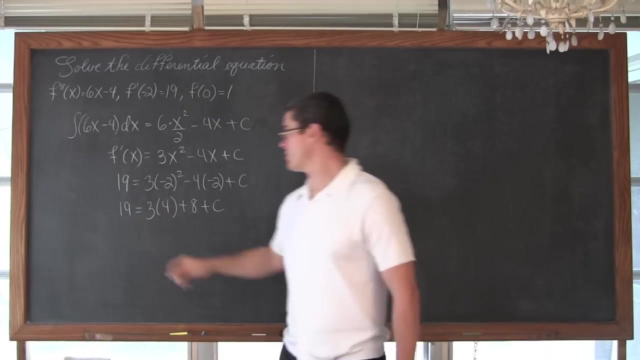 is equal to 19 when x is equal to negative 2.. So we have: 19 equals 3 times negative. 2 squared minus 4 times negative. 2 plus c, That gives us 19 is equal to 3 times 4.. Negative 4 times negative. 2 is positive 8 plus c 3 times 4. 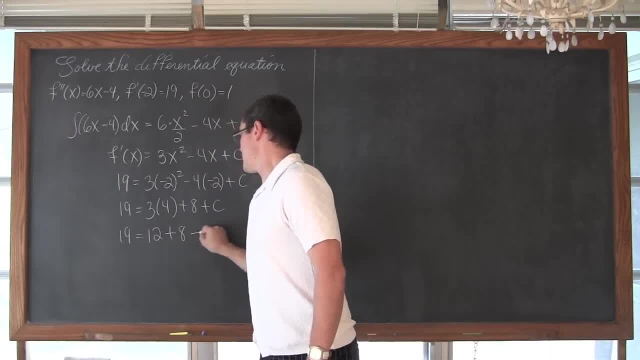 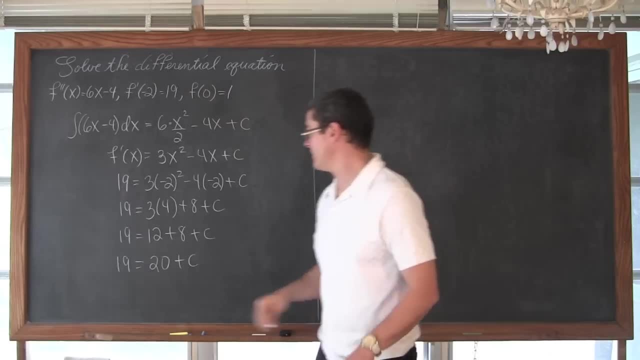 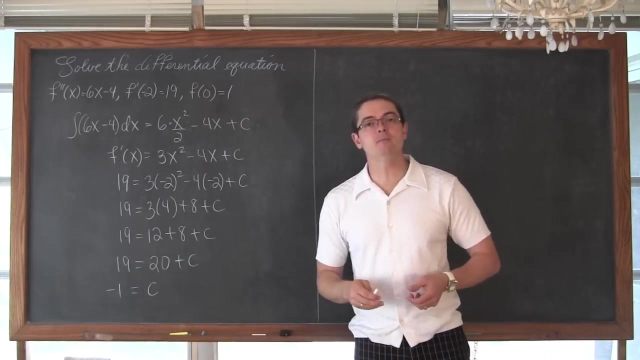 is 12 plus 8 plus c, That is 19 equals 20 plus c. Now when you subtract both sides by 20, you get negative 1 equals c. I am showing all these steps, of course, to help you better understand what I am doing. 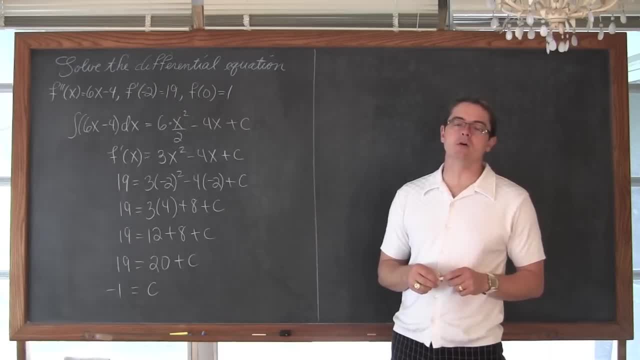 And also, as we are starting to learn, a lot of calculus problems are very long, So the more steps you skip, the sloppier you are with your notation, and your handwriting makes it much, much easier to make those small, niggly mistakes or careless mistakes that you know. 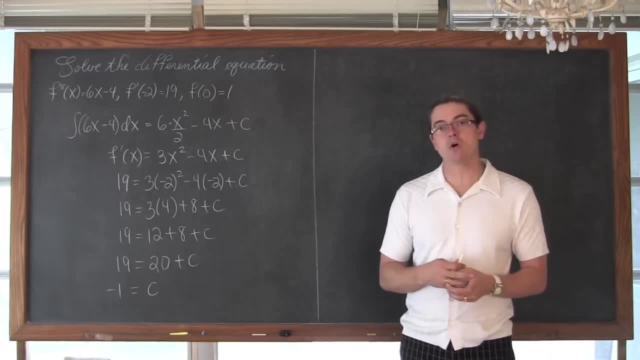 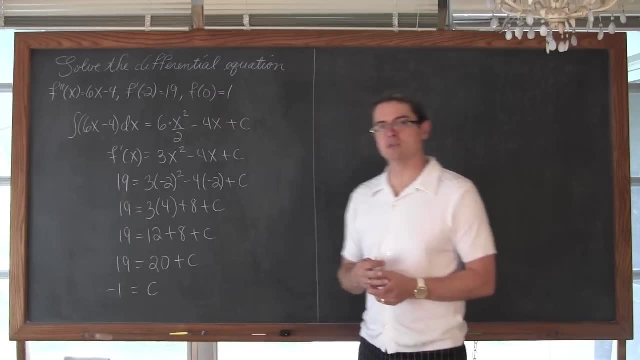 we get to the end. we basically followed the right processes, but our answer is wrong. So make sure you show those steps nice, clear and precise so that when you get done you haven't wasted all that effort to get the wrong answer because you didn't, I don't. 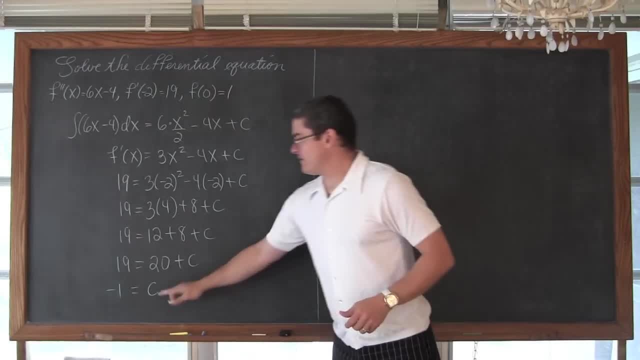 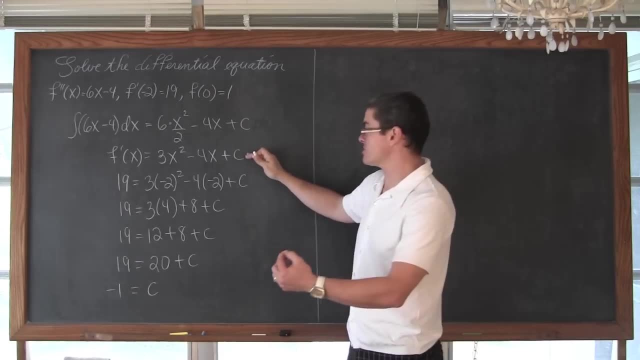 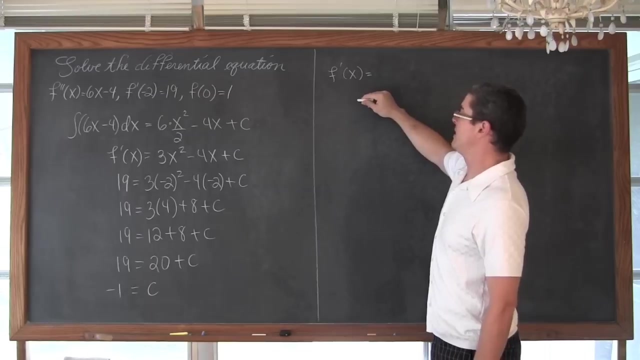 know 2 and 2 is 5.. Is that okay? So now that we have found that value of c, we can go ahead and plug that back into our general solution for the first derivative and find that particular solution. So coming up here we have f. prime of x is equal to, or the first derivative of f is equal to 3x squared. 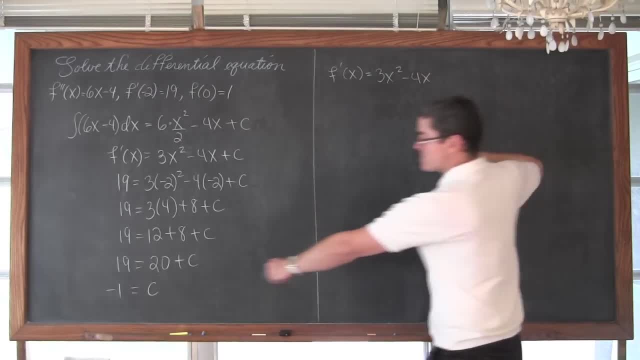 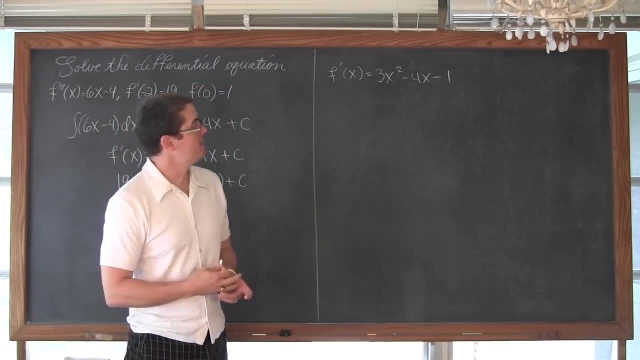 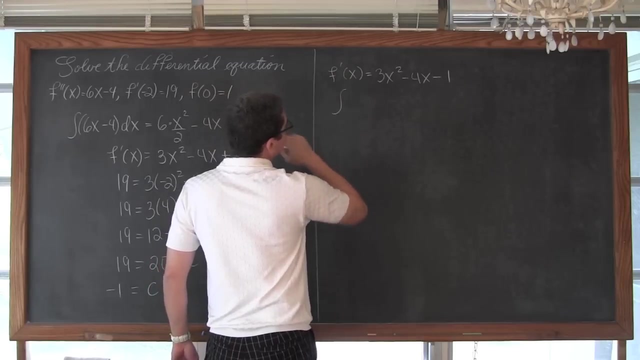 minus 4x, Now minus 1, because now we know what c is equal to. Ok, we are going to have to go through the antiderivative process again To 0.. general solution for the original function. So we are going to take the integral of 3x. 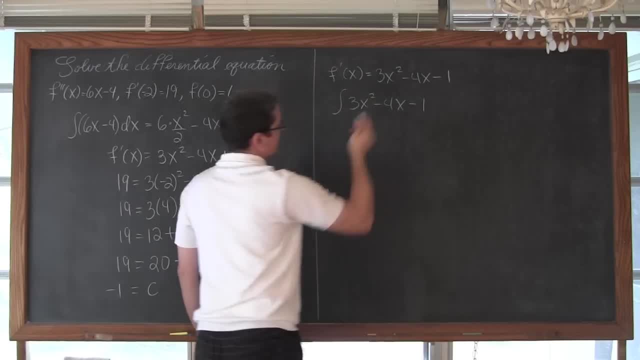 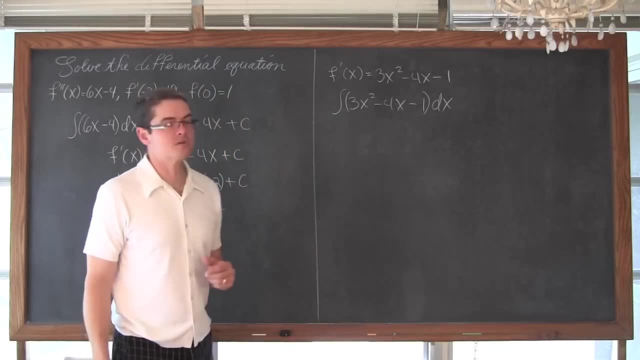 squared minus 4x plus 1, or find the anti-derivative with respect to x. Ah, yes, with respect to x. If it is easy for me to forget that, I am sure it is easy for you. Make sure you are. 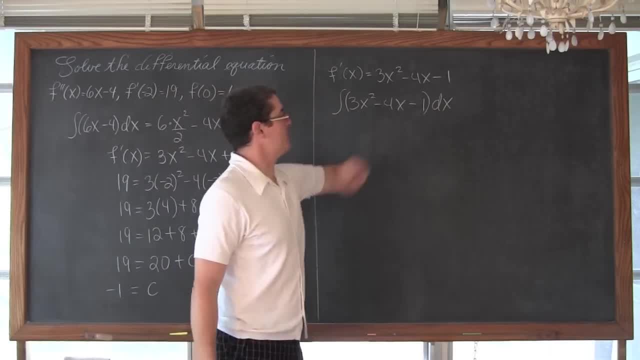 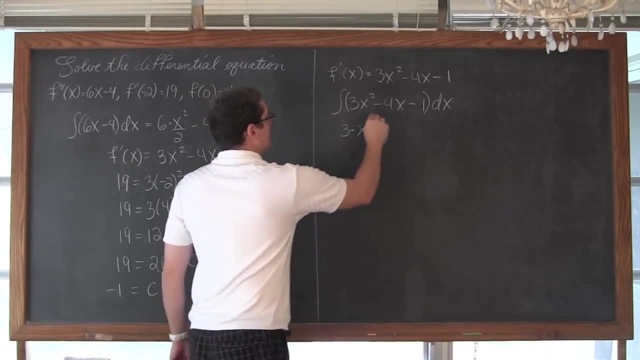 particular with your notation. Your teacher will not be happy if you keep forgetting that. So we are going to have 3 times x. We are going to raise that power by 1. And again divide that by the same value Minus 4,. raise that exponent by 1 and divide by the same. 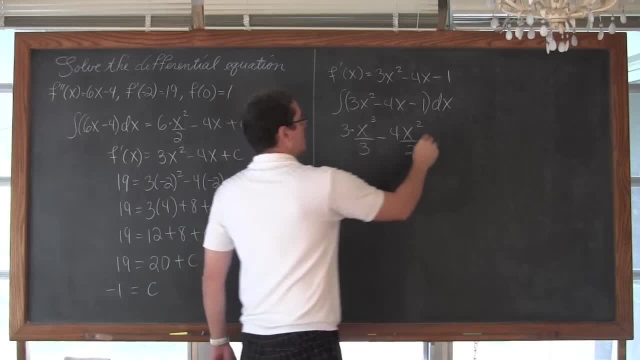 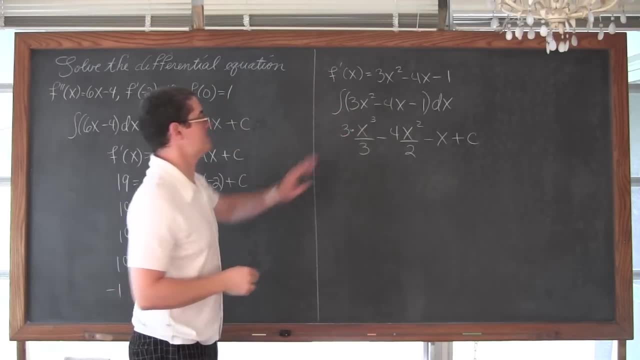 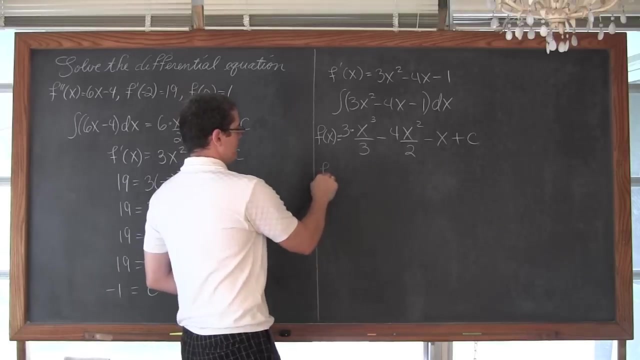 value, Just using that power rule with each of the individual terms: Minus x, plus c. Now this is the first derivative. We just did the anti-derivative, which now means this is our, we are going to be our- general solution for the original function. So f times x is: 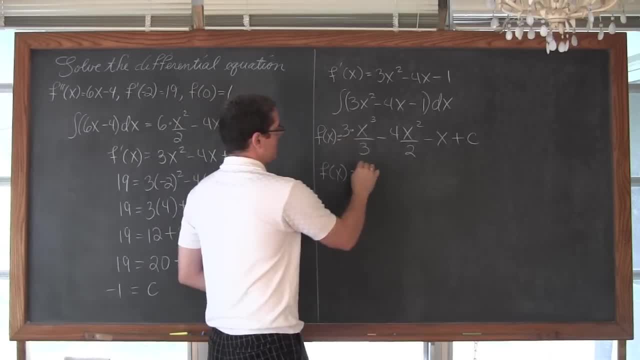 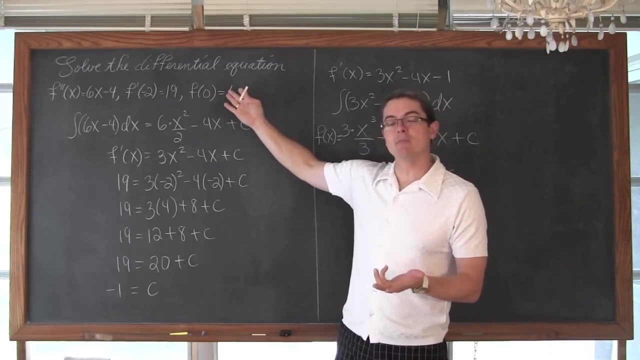 equal to 3 divided by 3 is 1.. So x to the third, 4 divided by 2 is 2.. So minus 2x squared, minus x plus c. And now we use the initial condition or this extra piece of information. 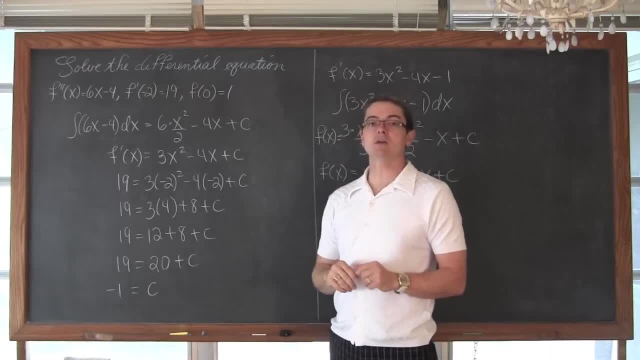 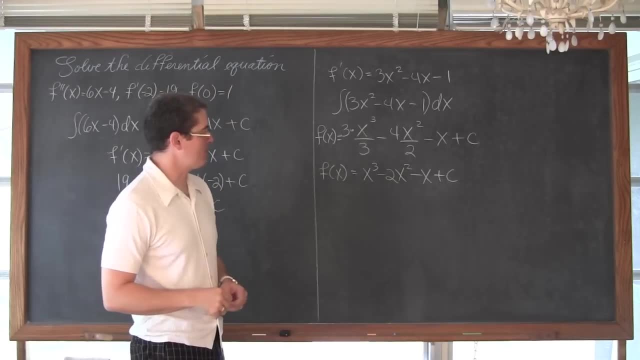 given to us about the original function That says, when you plug in an x value of 0, you get a y value of 1.. And I just thought, since this is a two part equation or a two part problem, I would be nice and give it a try.